bare soil, raindrops will not grow. If you have a lot of bare soil, raindrops will not grow. If you have a lot of bare soil, raindrops will not grow. If you have a lot of bare soil, raindrops will not grow. 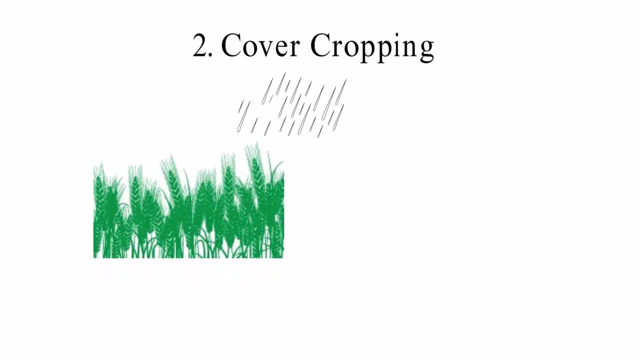 Cover cropping can help stop splash erosion. Cover crops can be grown between the main crops. They can give crops the nutrients they need Most. cover crops make the soil nitrogen-rich. This farming method can also make the soil better able to hold water As a result. 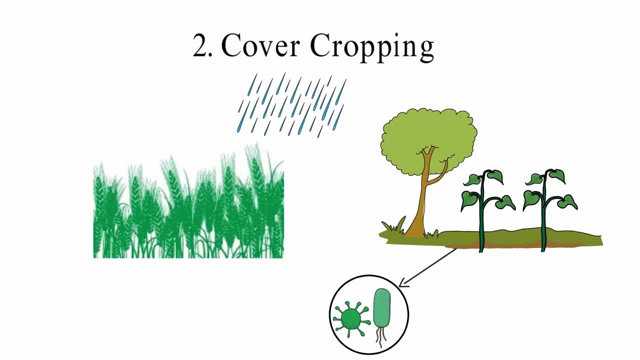 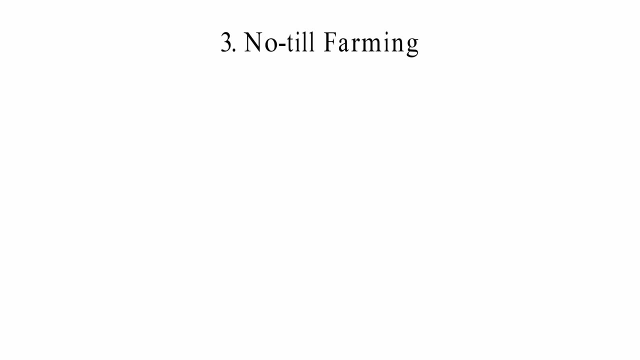 they give soil microbes the right conditions, which improves soil fertility. This also means that farmers can use cover crops as animal feeders. Cover cropping can help stop splash erosion. 3. No-till farming: No-till farming is all about protecting the soil from being disturbed. 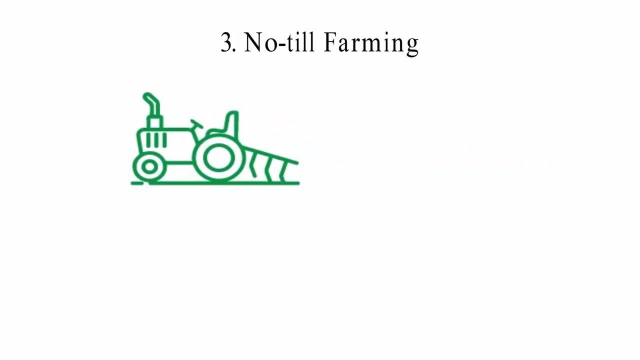 Tilling can have a number of effects on the soil. It can cause water to be lost and also destroy plant cover. Tillage that goes on for a long time can make the land look very dry and empty. This can cause soil to be lost and nutrients to be lost. People who grow crops 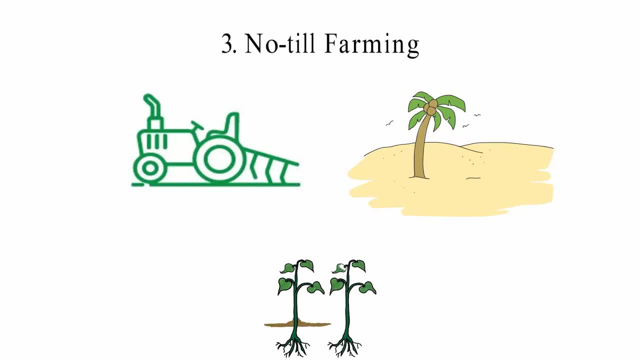 can help save soil by planting cover crops. 3. No-till farming: No-till farming is all about protecting seeds in the crop residue. This will not only cut down on the cost of framing, but also keep the soil structure. No-till farming also stops runoffs. There won't be any soil nutrients lost when it. 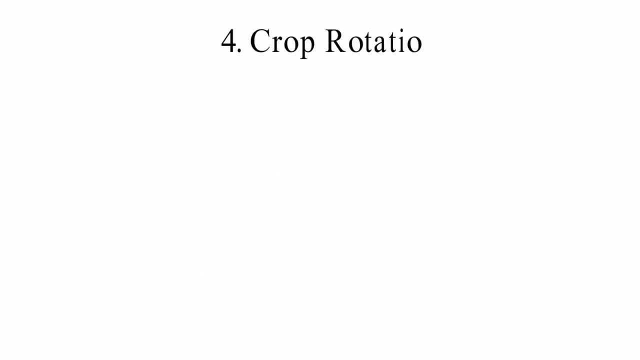 rains, so that won't happen. 4. Crop rotation: Crop rotation is a farming method that lets you grow a lot of different crops on the same piece of land at different times of the year. If you want to improve the soil, for example, you can plant leguminous plants like beans and corn. 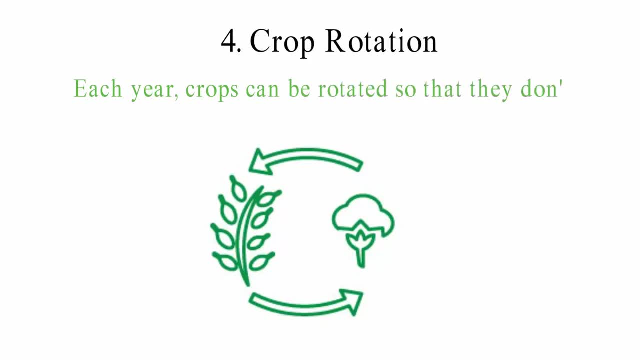 together in a row Each year. crops can be rotated so that they don't need to use fertilizers and other farm chemicals. It takes a lot of planning to use this soil conservation method To get the best results. farmers need to pick the right plants to rotate with, Because different crops 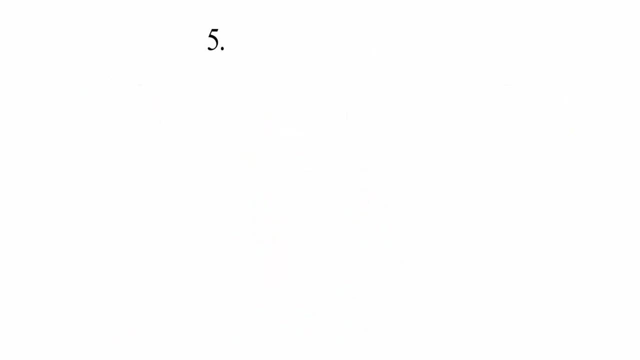 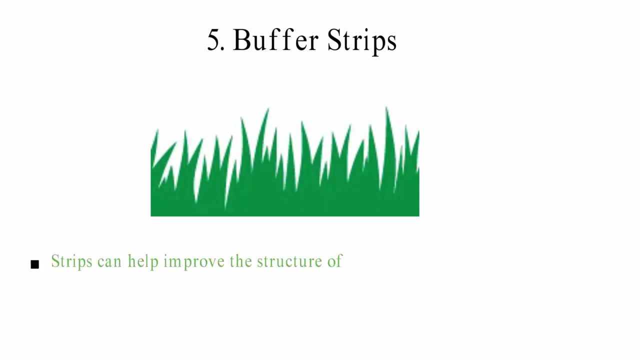 used for farming. Strips can help improve the structure of the soil. Also, buffer strips can help slow down surface runoffs. Roots of buffer strips hold soil particles together and can keep them from moving when it rains. Buffer strips can also stop wind erosion by protecting the land from 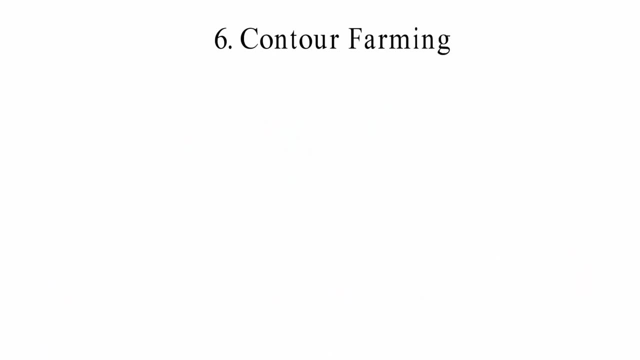 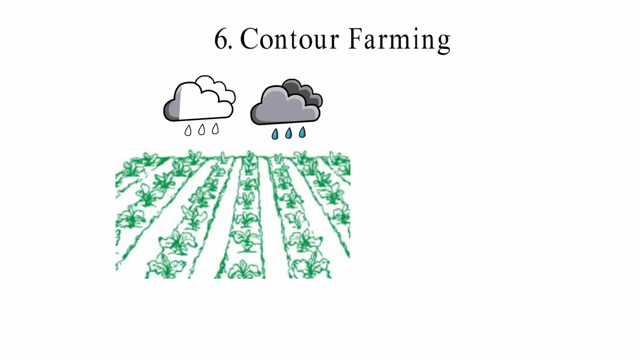 the wind. 6. Contour farming: If you want to make your land look better, you can terrace it, but contour farming doesn't change the shape of the slope. This type of farming asks farmers to make a lot of rows of soil along the contour. When there is a lot of rain, rainwater won't. 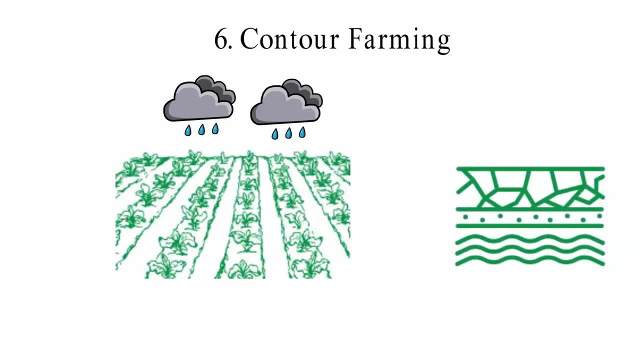 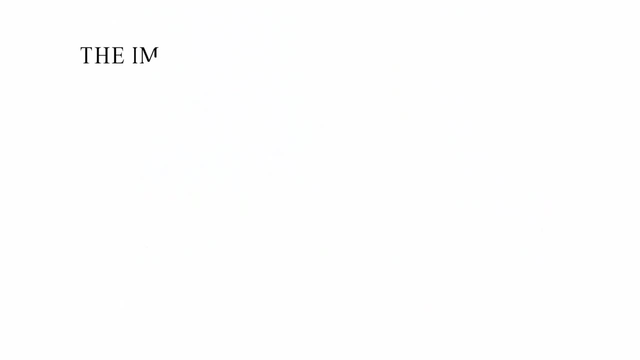 be able to flow. downhill Contour farming helps protect the soil from possible erosion and other types of soil damage. Runoffs are less likely to happen in landscapes that are shaped. Soil nutrients will be kept as long as possible by this method. The importance of soil conservation. In order to improve the soil, you need to keep the soil in. 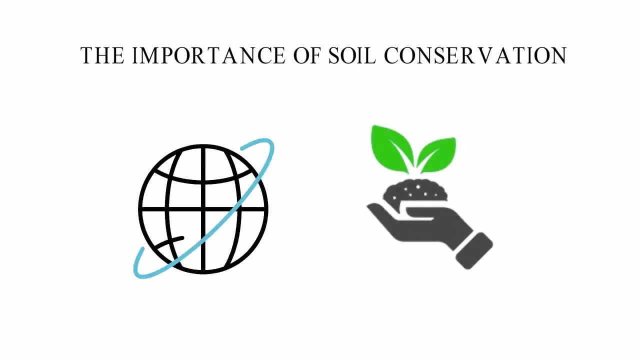 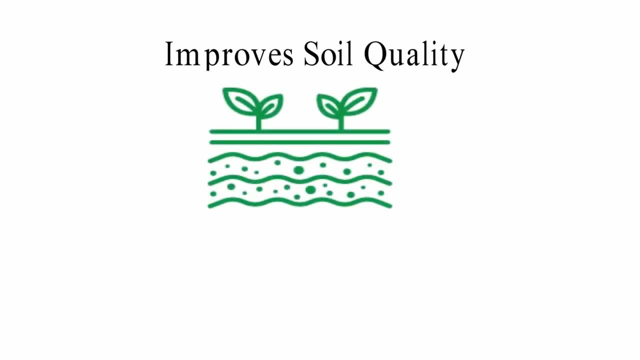 good shape. It's not just good for the soil but for the whole world. Improves soil quality. Soil conservation improves the structure of the soil, which makes the soil better for us to live on. Well-maintained soils tend to be more fertile. 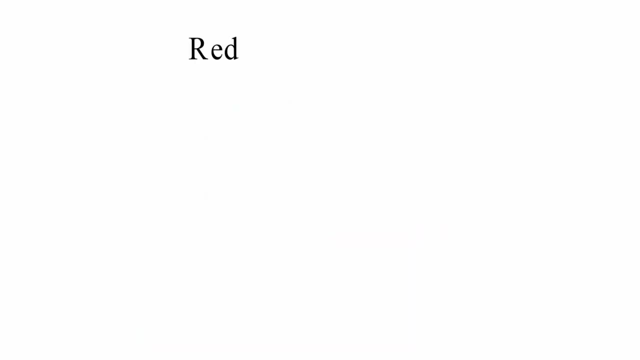 Which means more crops and lower farming costs. Reduce soil erosion. The farming methods used in soil conservation can help stop soil from being washed away. Most of these things give the soil more protection from wind and water. Improves water infiltration. It can hold more water when the soil is good at filtering. 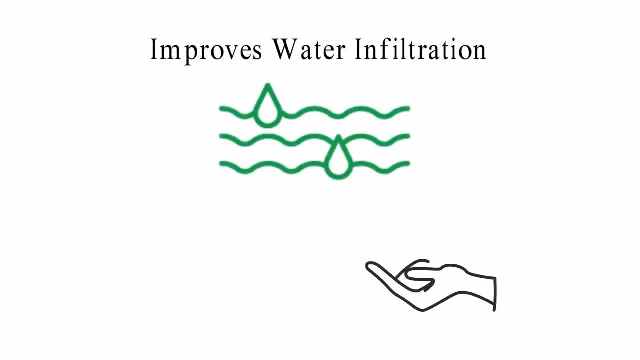 so it can hold more water. The crops will have everything they need to stay healthy. 7. Contour farming: If you want to make your land look better, you need to keep the soil in good condition, as long as there is good filtration, Soil microbes, like wet conditions. This means that 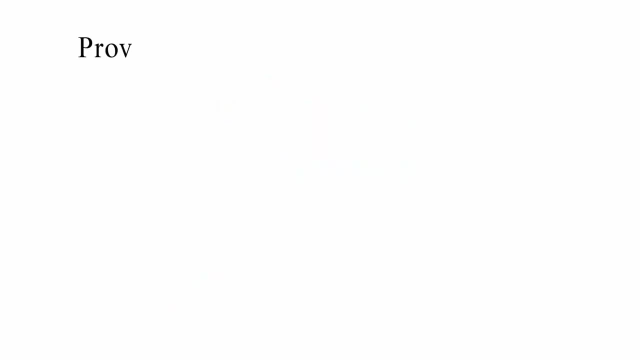 the soil will be more fertile when there is good drainage Provides animals with food and shelter. When we take care of the soil, we can grow more plants that animals like to eat. A lot of livestock can get food from cover crops. Animals can also hide. 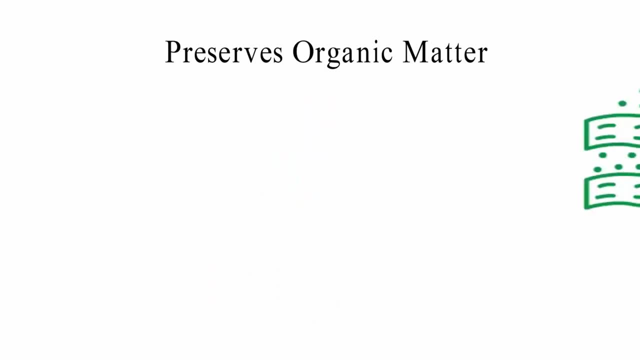 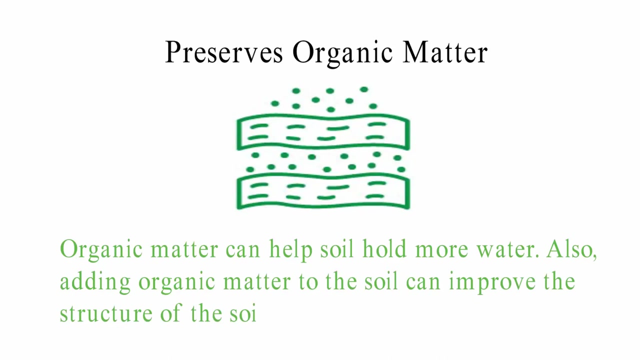 from the sun under vegetation cover Preserves organic matter. If you keep your soil healthy, you could have a lot more organic matter in your soil. Organic matter can help soil hold more water. Also, adding organic matter to the soil can improve the structure of the soil. 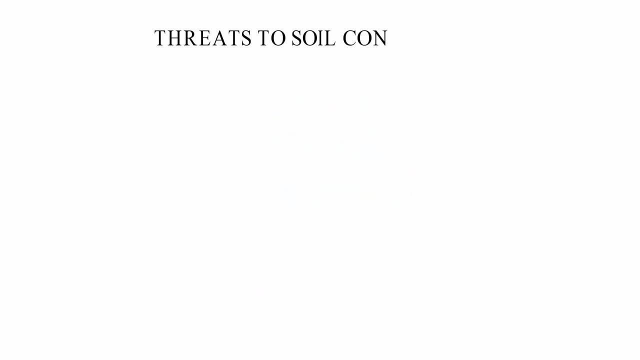 Threats. Threats to soil conservation. The main threat to soil conservation is poor farming practices. This can result from: 1. Overcropping. Overcropping can happen when a lot of tillage takes a toll on the soil. It can causeulture decay. Overcropping can cause a lot of soil decay. 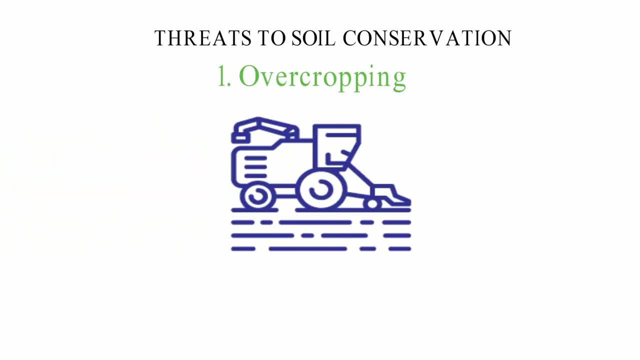 Overcropping can cause a lot of soil decay. Overcropping can cause a lot of soil decay. The most public access to organic soil is by combining organic soil geraunification and organic soilliga containing toll on the land When the same types of crops are grown on the same piece of land over and over. 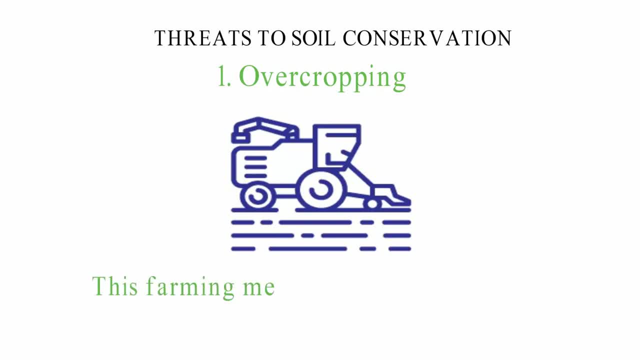 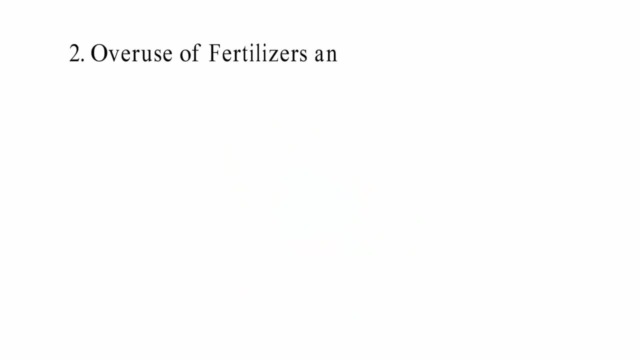 again, it can make the soil less healthy. This farming method can also lead to the loss of nutrients in the soil. 2. Overuse of fertilizers and other farm chemicals. Farm chemicals can damage the soil. When herbicides and pesticides are used over and over again, they can get into. 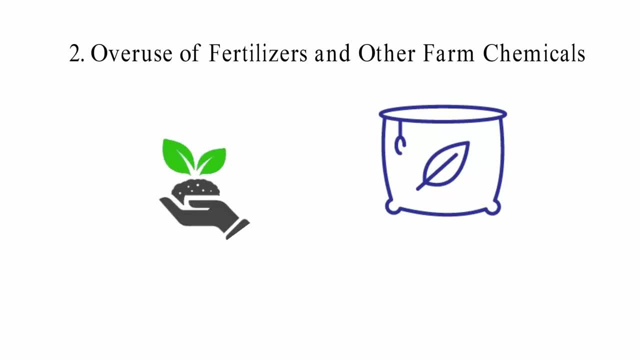 the soil. Too much fertilizer in the soil can change the soil's pH. This can make the soil less acidic. This can kill soil microorganisms and plants and it can also hurt them. 3. Slash and burn farming practices. Slash and burn is a way to remove vegetation cover from a piece of 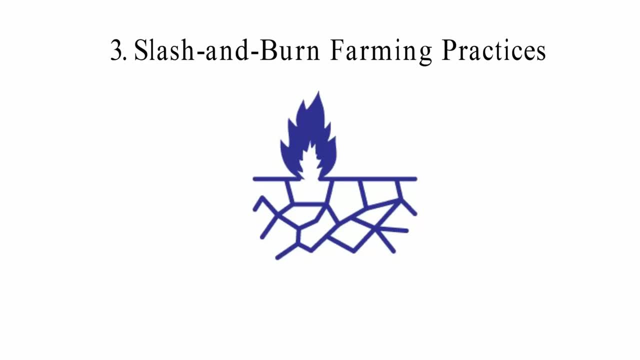 land by cutting it down and setting it on fire. This can be done when the land is ready for tillage. It can eat away at the soil. It can eat away at the soil. It can eat away at the soil. It can eat away at the soil's humus and make it dry out as well. 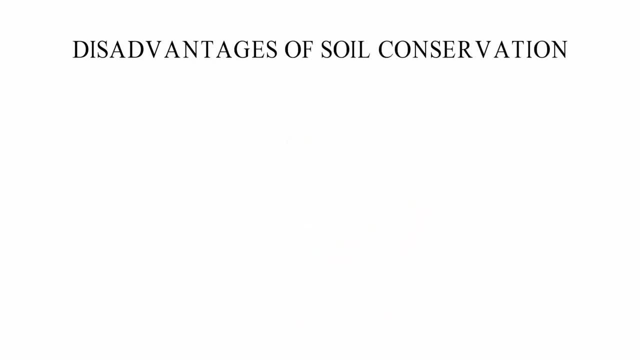 Disadvantages of soil conservation. Certain soil conservation practices may cause problems during or after planting crops. Using the no-till farming method can make it a little more difficult to plant because the seeds won't fall on the soil all the time. This can make it more difficult. 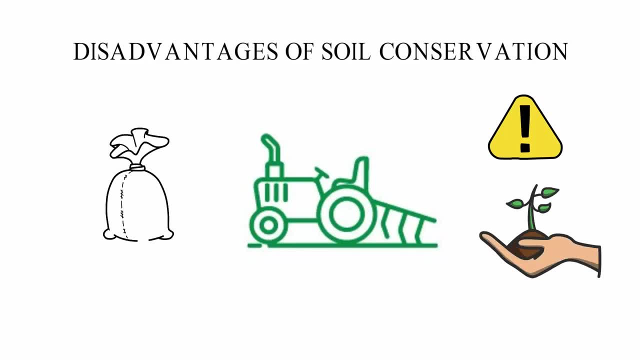 This can stop the seeds from growing. It can cost more to grow food if herbicides are used instead of fertilizers. This can make it more difficult to grow. This can stop the seeds from growing. This can stop the seeds from growing. This can stop the seeds from growing. This can